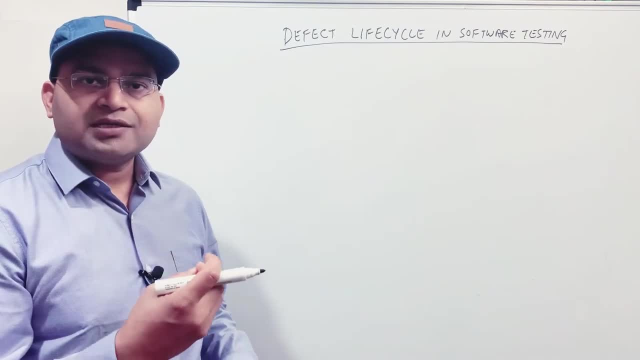 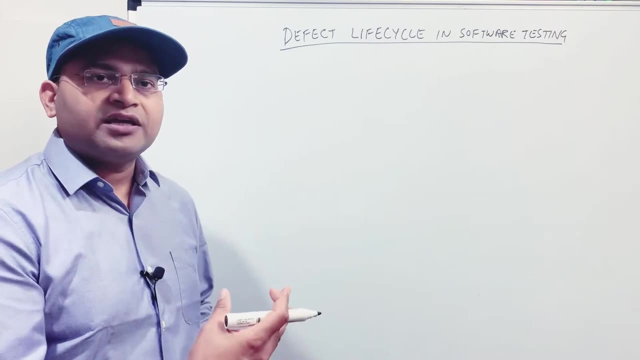 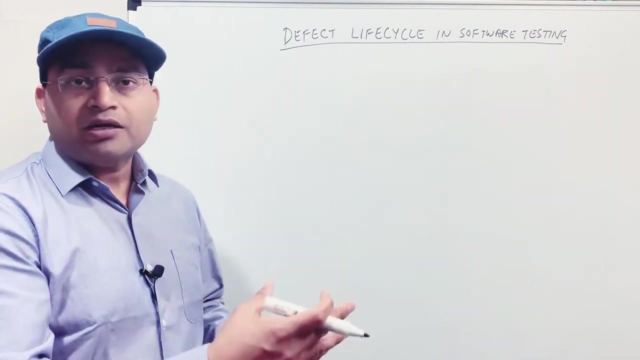 you are trying to contact any customer support. say, you have bought a phone and you have got some issues on your phone and you want to clarify certain doubts and you have raised a ticket with a customer support department of that particular company. So what you usually do, you pick the form or you basically 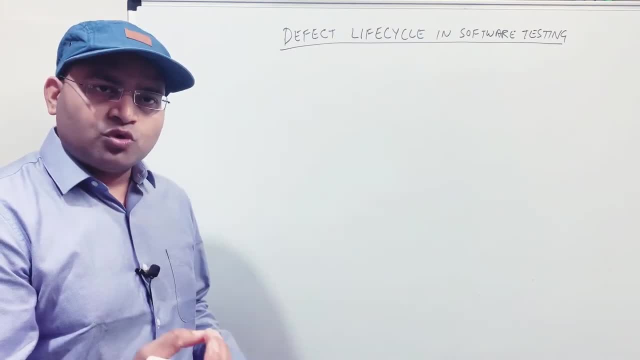 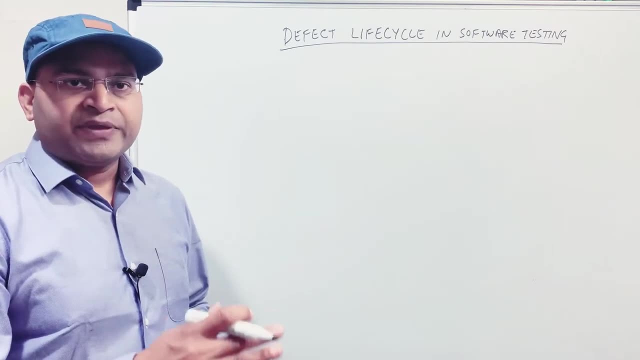 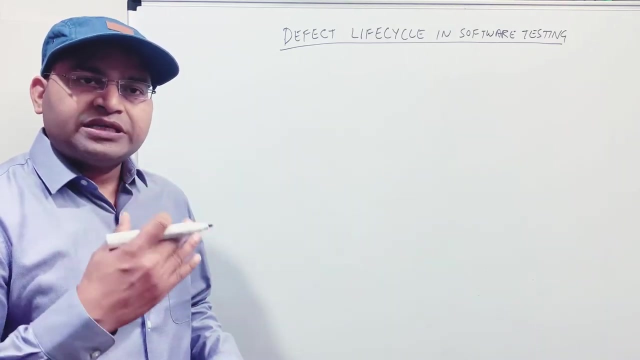 go to the website, click on support and then they have the support form. You provide all the details and then submit the application or submit the ticket. Then that ticket goes into the backend and follow certain process. right, So they'll reply to you So once you raise. 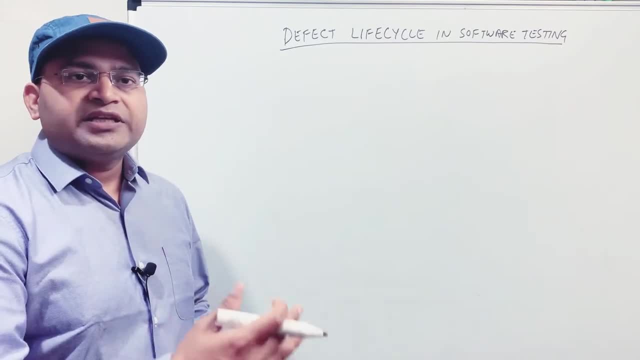 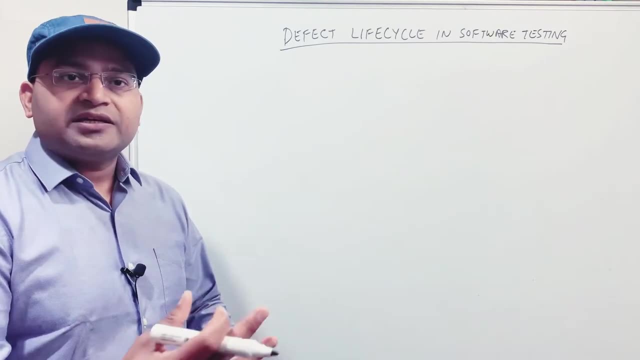 the ticket. it's basically a new ticket for them. Then if they need any information, they'll assign it back to you and you need to provide certain details. So this is the case of any ticket that you raised in the customer service department. Now, when we talk about the defect life cycle, 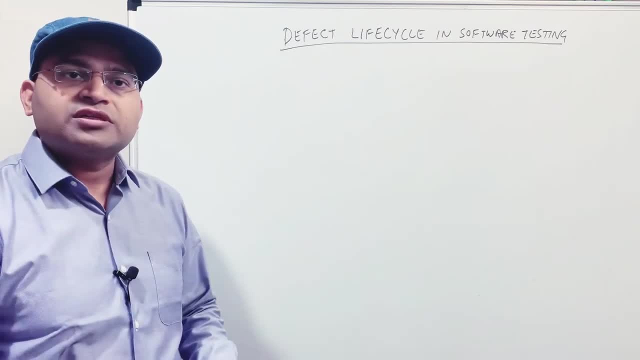 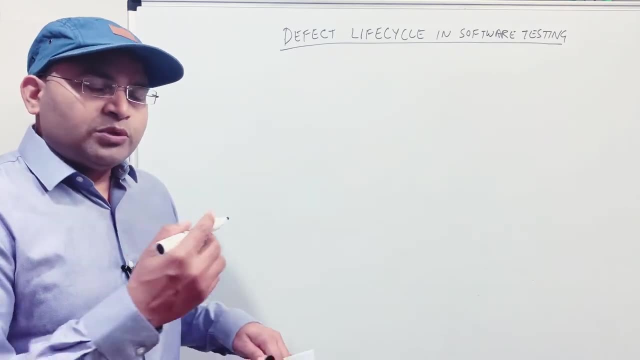 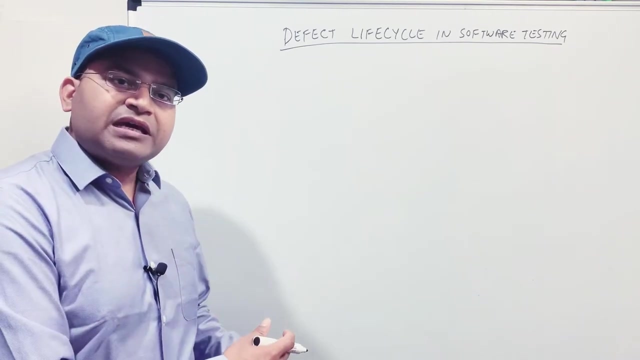 so the life cycle of defect will follow certain, something similar to what we have done in case of customer service. so when we say defect life cycle, it's basically the life cycle of the defect in software testing project. the example that i gave for the customer service is the life cycle of the 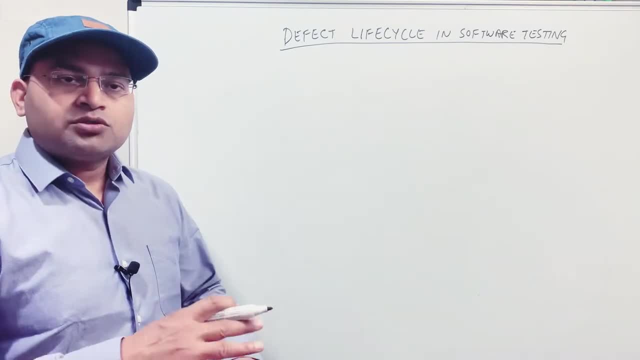 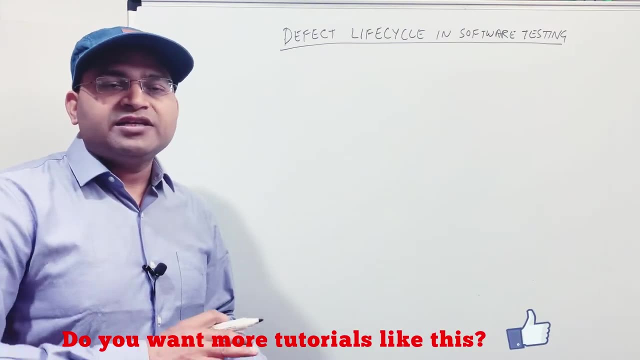 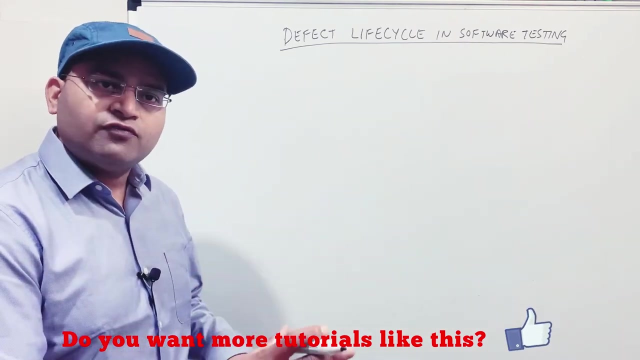 issue or the support ticket that you raise, right? so in terms of life cycle, understanding of the life cycle, it's same. it's basically the process that an issue will follow. it's the customer service life cycle and, when we talk about the defect, a process that a defect will follow in. 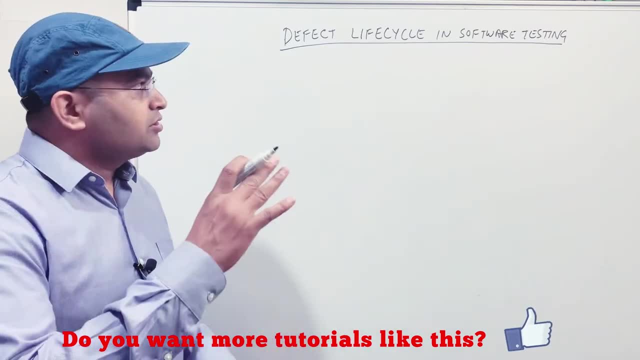 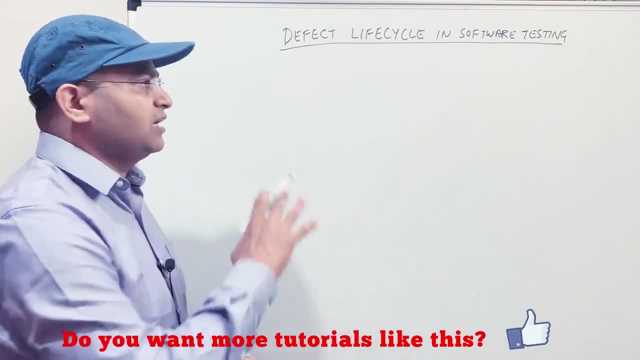 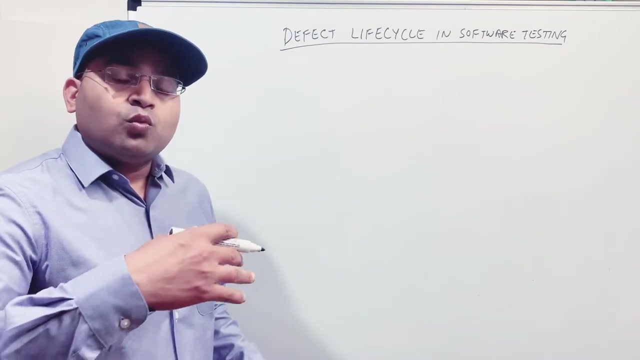 software testing project. is defect life cycle right? so that's a brief about a defect life cycle. i hope that this analogy will clarify a lot of your doubts around the defect life cycle or what exactly defect life cycle is. now the next thing is: what are the important statuses and how the 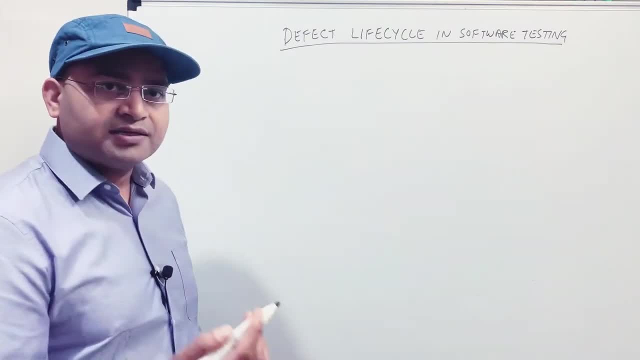 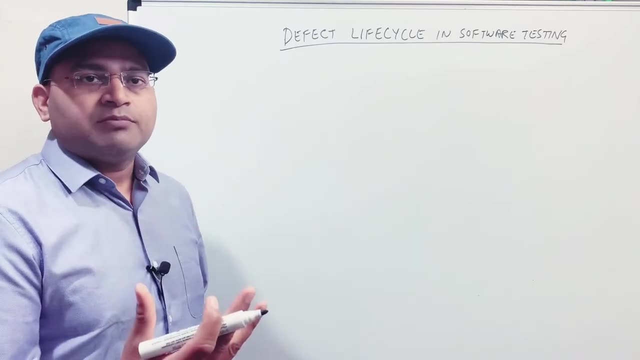 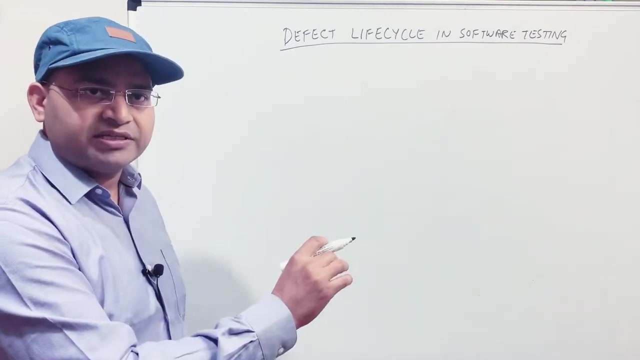 defect life cycle looks in software testing. so the first state you should usually will be: if you found a defect, you will be raising a defect. so to raise a defect in the defect management tool, you will launch the application or you launch a defect template or defect form and you will provide all the details and submit the ticket, right or submit. the defect. once you submit the defect, the first state is the new state of the defect right, so that's a new status. once the defect is in the new state or the new status, usually the- the good practice is that within the new status itself you will have the defect triage meeting. and in defect triage meeting what happens is: 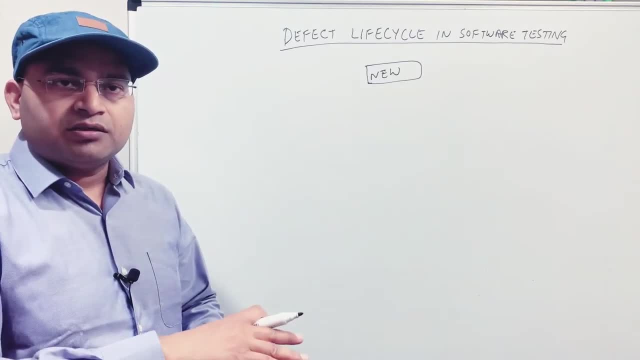 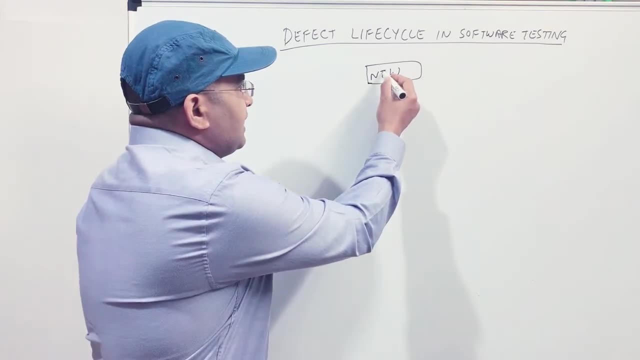 uh, the, the development manager, test manager and uh- mostly the person who has raised the defect, or a couple of people from the uh testing team, will have a meeting and they'll go through and analyze the defects that have been raised. say, for example, your test team is big. there are a lot. 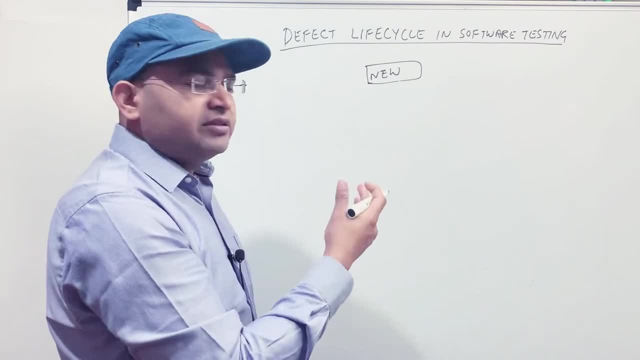 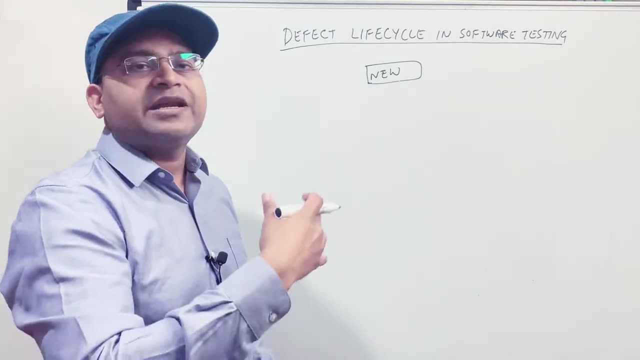 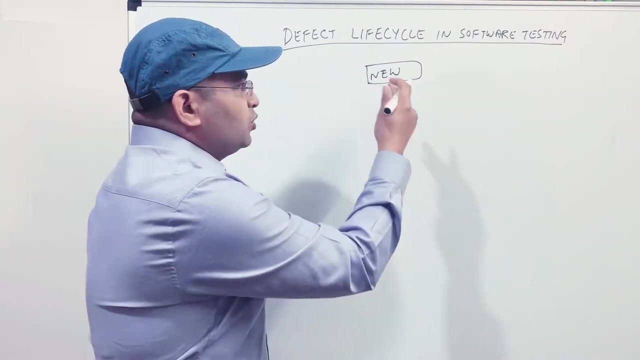 many defects being raised. they'll analyze the defect and they'll, based on the analysis, they will identify whether the defect need to be fixed now or it can be deferred. if say, for example, defect is not very uh, not on high priority, then they can say we don't want to fix in this particular sprint. or 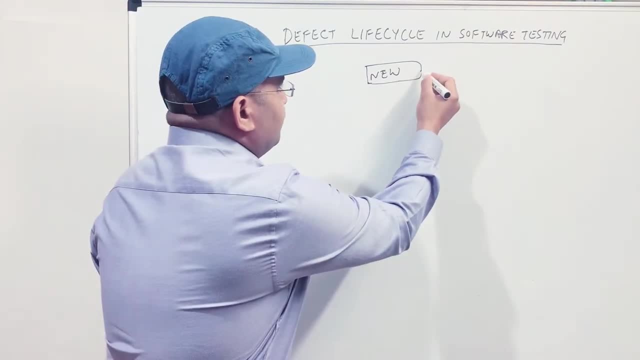 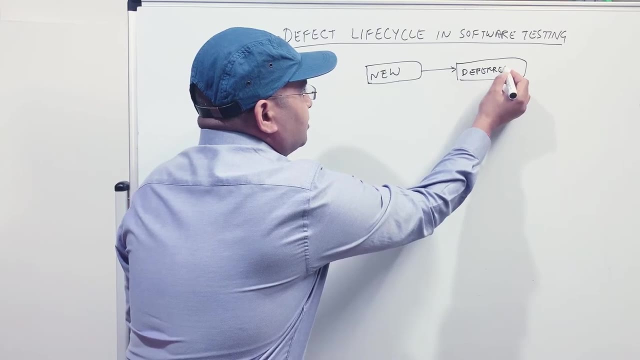 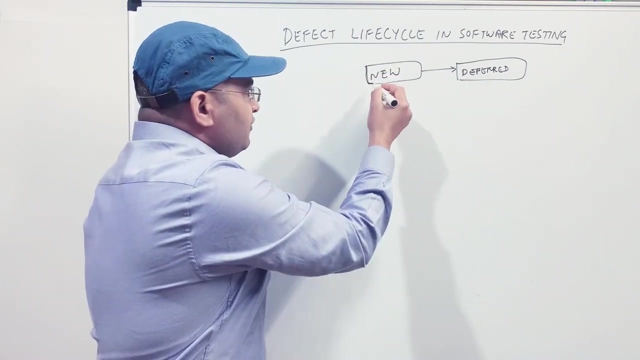 in this particular release, we can defer it. okay, so from the new state the defect can go to the deferred state. right, so that's another status. so, based on the defect triage, it can move to the deferred state now if, within the triage, out of 10 defects, two have been moved to deferred and eight have been. 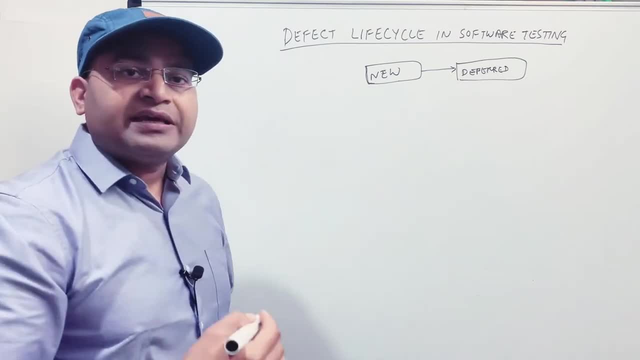 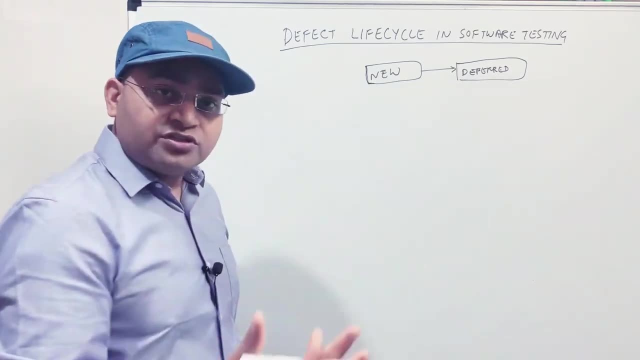 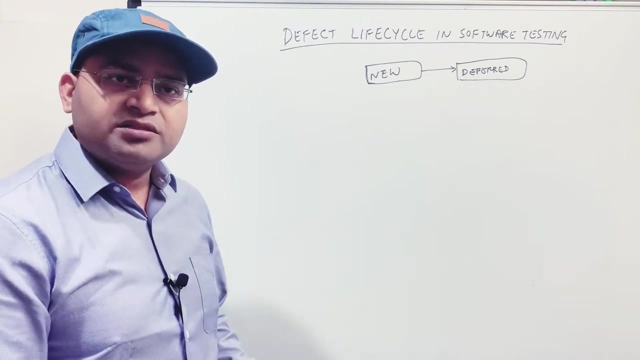 accepted right. so if the eight defects have been accepted, the next status is to assign those to the person who will work on those right. so who will fix those defects? developers will fix those defects. so now, after the new state, after defect triage happens, the development manager will basically. 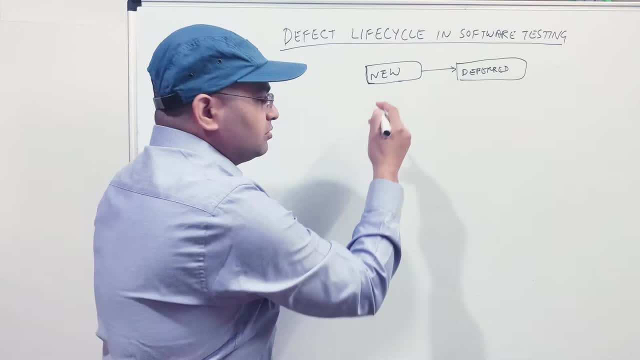 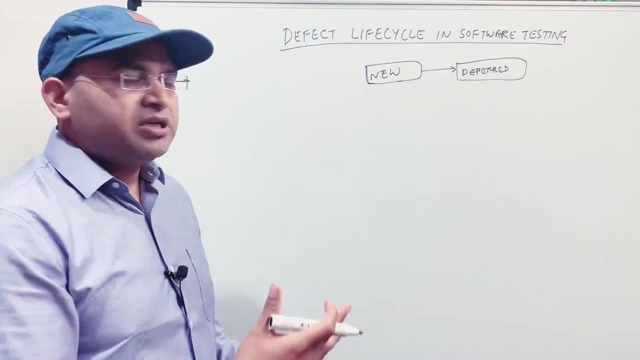 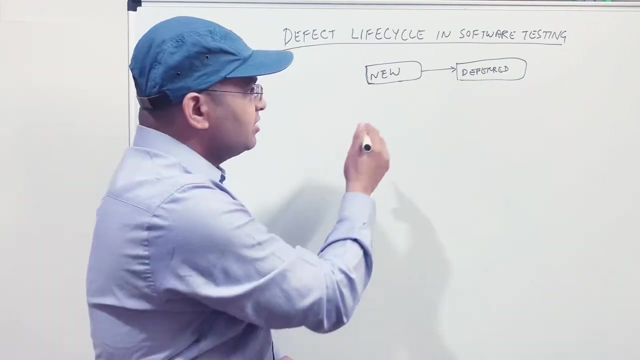 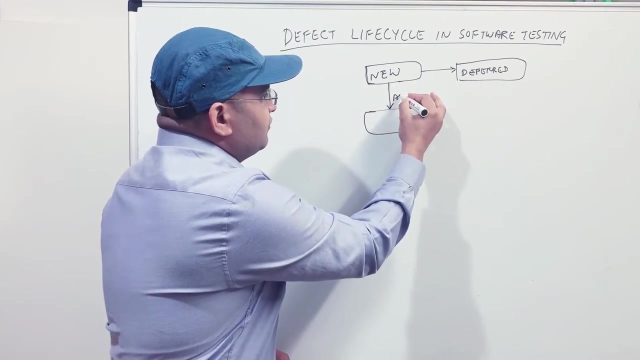 uh, assign those defects to the developers if it is, you know, a big team or, in case you are, a small team, within sprints. so you can, directly after having a discussion with the developers, and if, if the defect has been agreed, you can also, as a tester, assign it to the developer. and once the defect is assigned from, 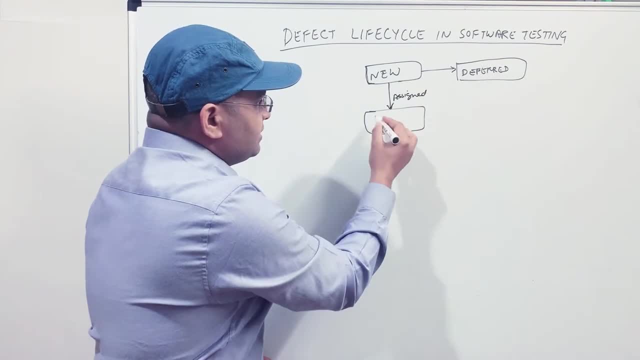 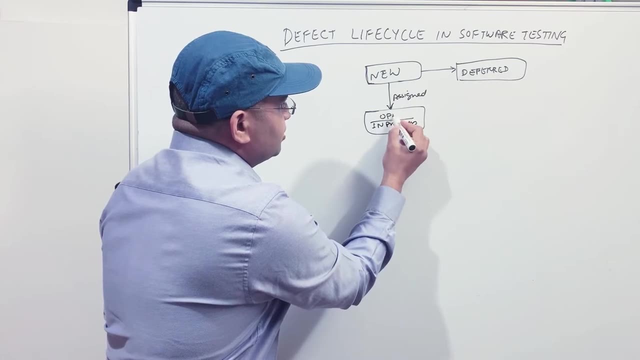 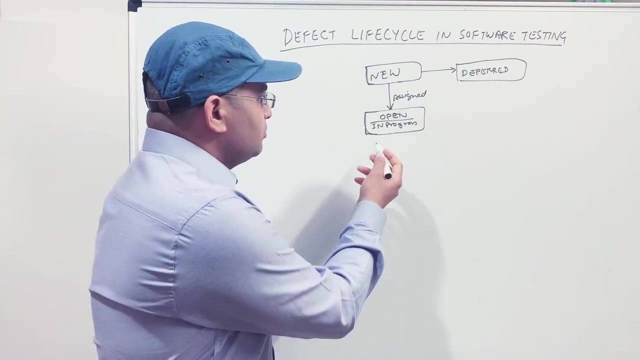 the new state, so from the new state it is assigned. the next state will be either in progress, so it depends what has been used in the tool, or it could be open, so from new it could be open, or in progress, right, so? so now the developer will start analyzing the defect once it is. 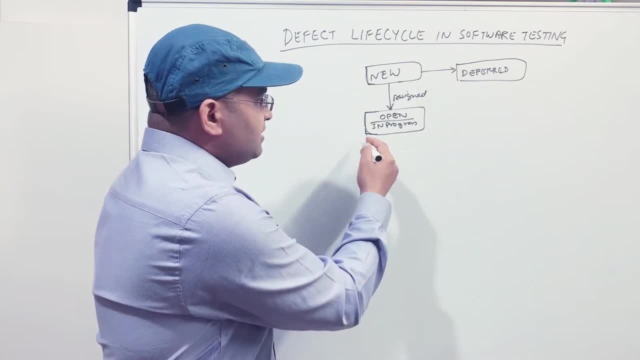 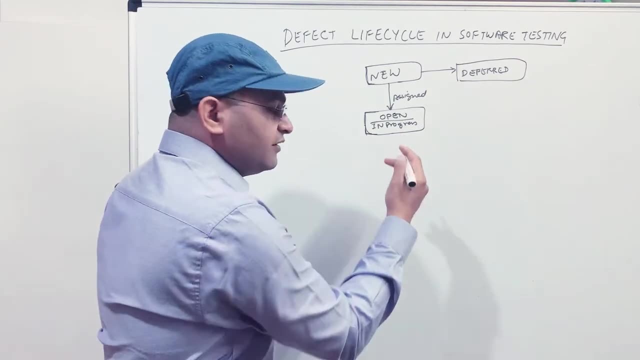 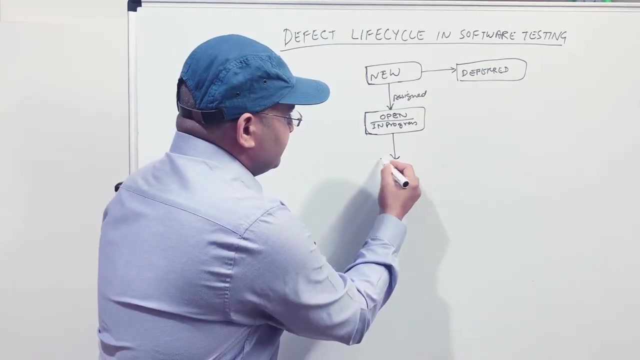 assigned to the developer and, based on the analysis, if he finds that, yes, it is the coding issue, he'll start fixing it. he'll fix it and once the defect has been fixed and deployed into the test environment for retesting, he will mark it as fixed. okay, so that's another state. 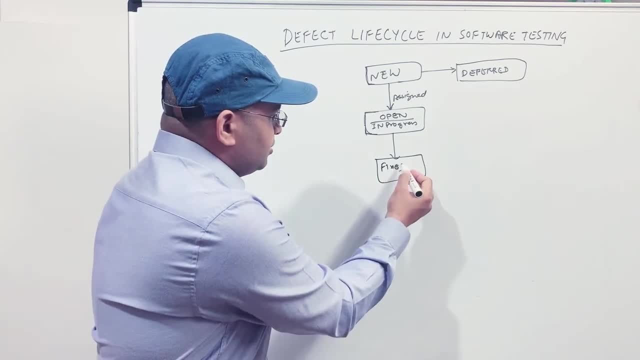 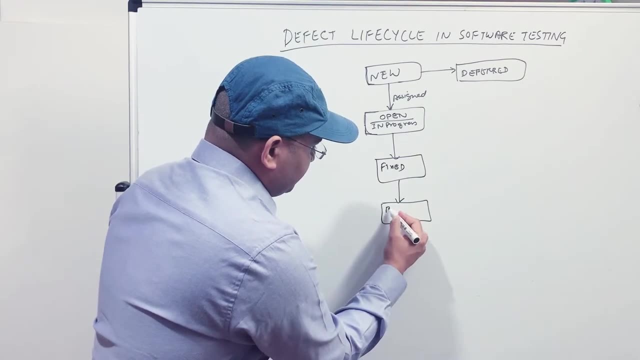 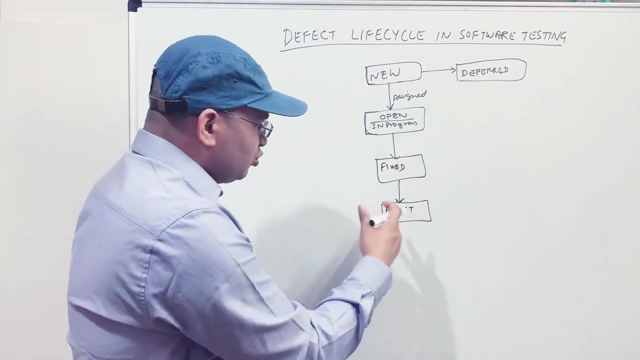 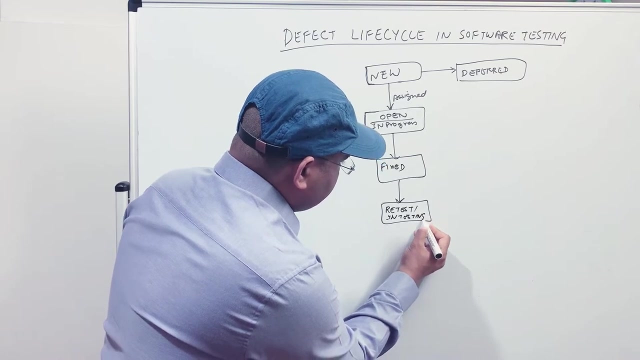 once the defect has been fixed and marked as fixed, the test manager will mostly move it to retest. right? so that's another state. so they'll reassign to the tester and they'll move it to retest, or it could be in testing as well. all right, so these statuses are customizable, so based on 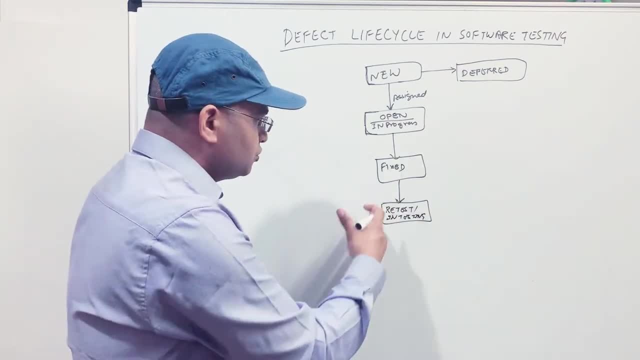 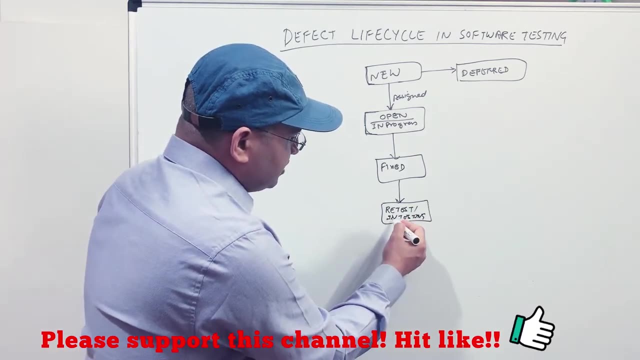 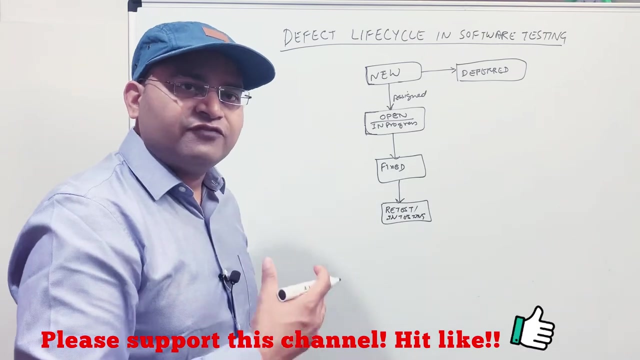 your project needs how the organization wants to use these terms. they can use specific terms. okay, so once the defect is in retesting or in testing and you are verifying the defect, if the defect has been successfully fixed, after your testing you found that the functionality is working fine. there are no more different if defect has been successfully fixed, which means that your default can now push to fit at the test tool. if you can tell me the functionalities that are still there cannot be done. so the problem in which the method is work well enough and it does not work well enough, so you have to useyinelift and you know, and you have open test and you have to have the smaller神 algún. 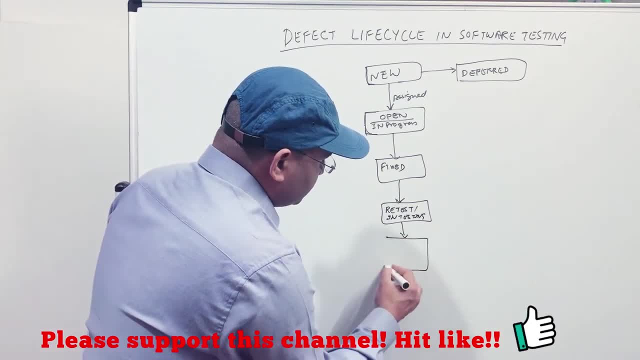 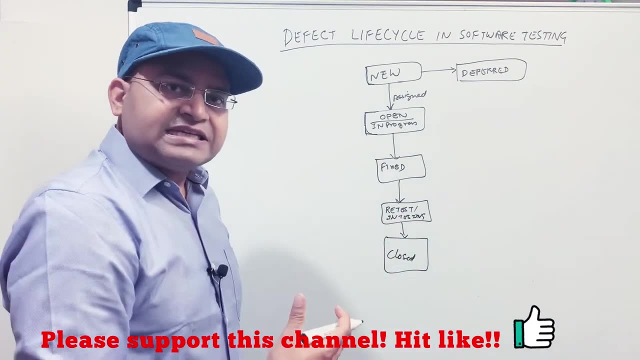 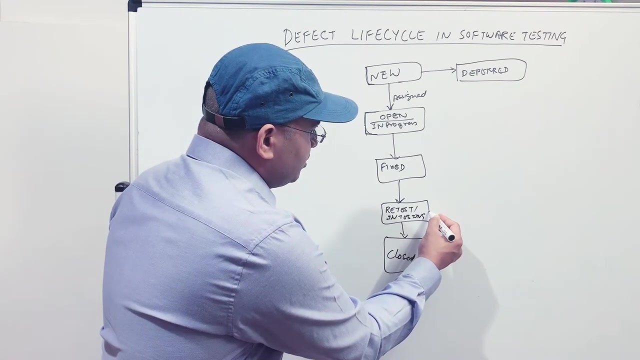 fact, onion perfect, since you, without having to use each other, etc. there are no more issues. then you will close the defect and the last state will be closed right in case the retest failed. so you are retesting the defect and the retesting failed, then you, what you will do, is you will reopen the defect right, so that 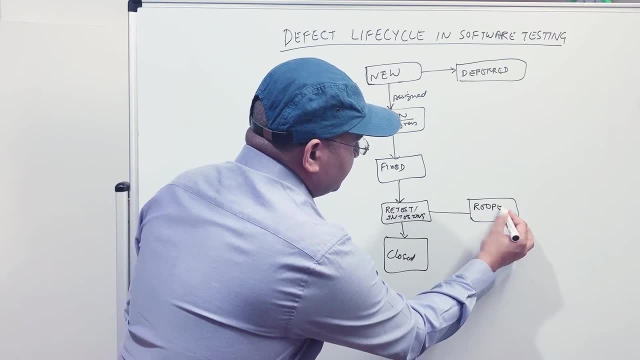 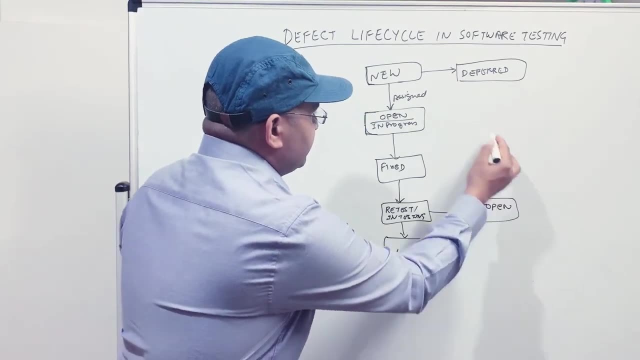 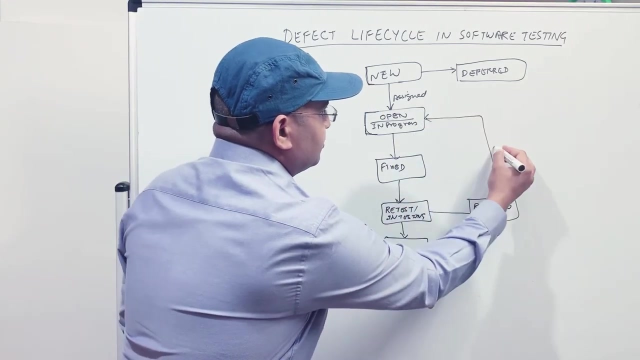 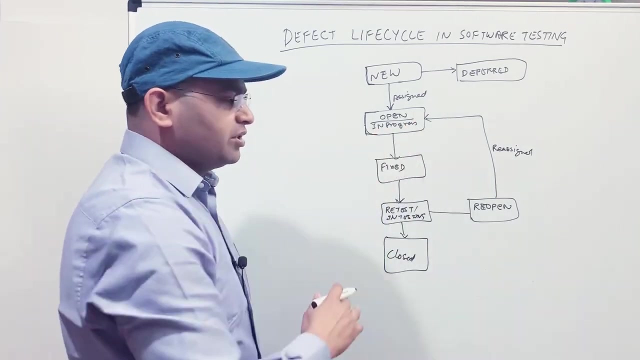 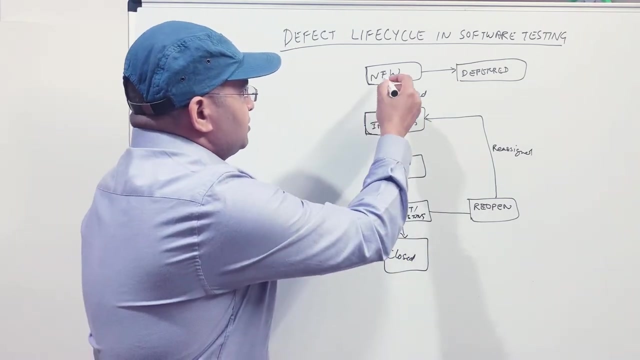 will be another state, so reopen. once the defect has been reopened it needs to be reassigned back to the developer to fix okay. so from reopen it will be reassigned and move to again to open state or in progress state. right. so this is how the normal flow of a defect will look like now. say, for example, the defect is in new. 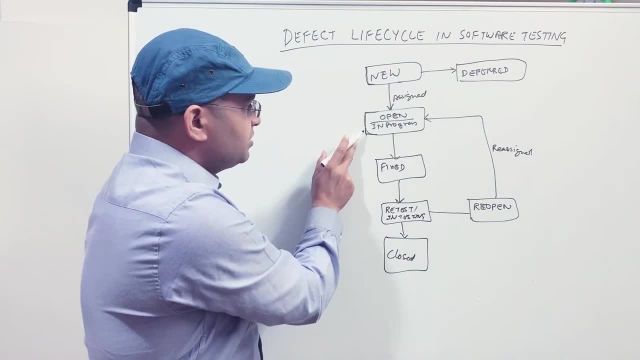 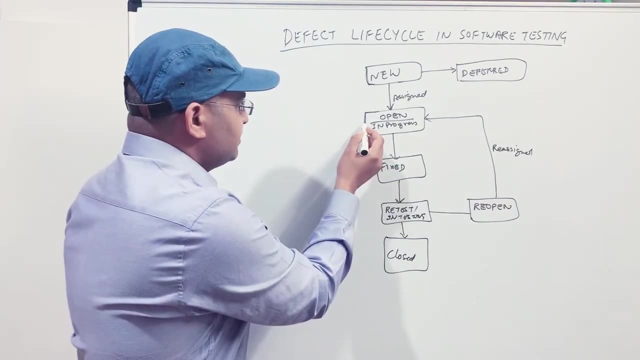 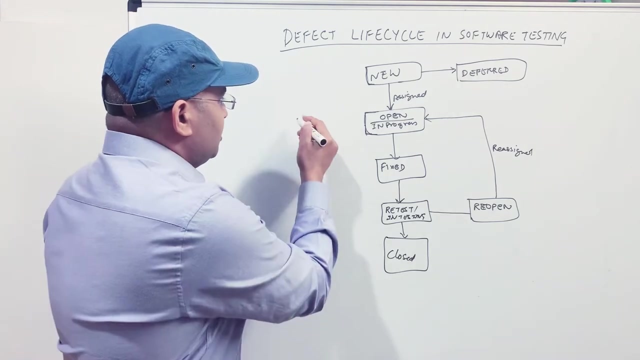 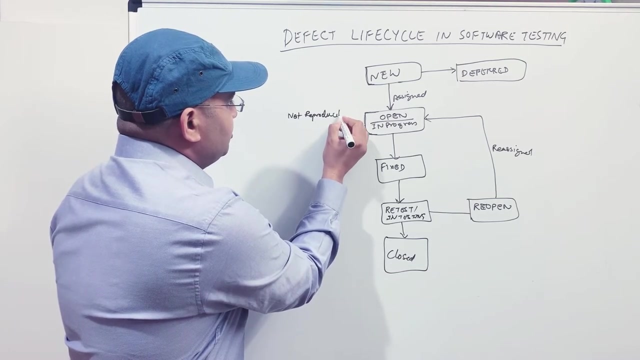 state it assigned. it got assigned to the developer in open state and in progress state. if, during the analysis, the developer found that this defect that he has been assigned to is not able to reproduce- he is not able to reproduce- then in that particular case what he'll do is he will assign or he'll say: not reproducible, okay. 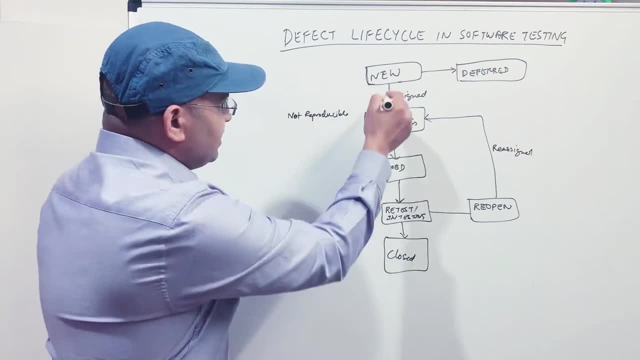 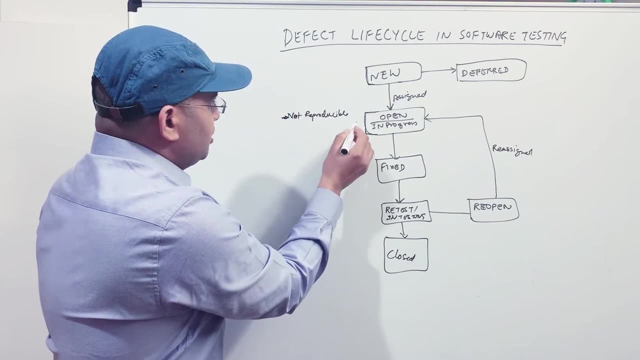 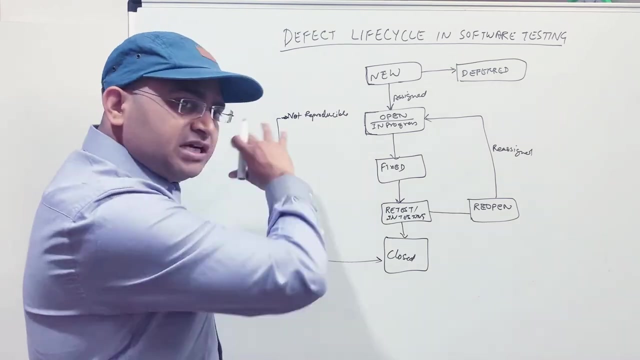 so this is the, these are the statuses and these, this is the resolution. so what he'll do is he'll mark the resolution as not reproducible and move the defect to closed from there. okay, there can be multiple scenarios, there can be multiple reasons. not reproducible is one, then the other could. 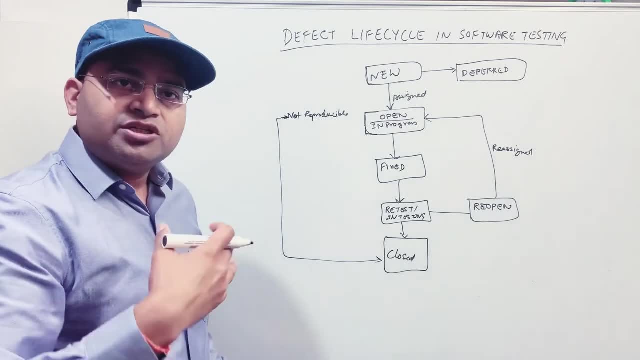 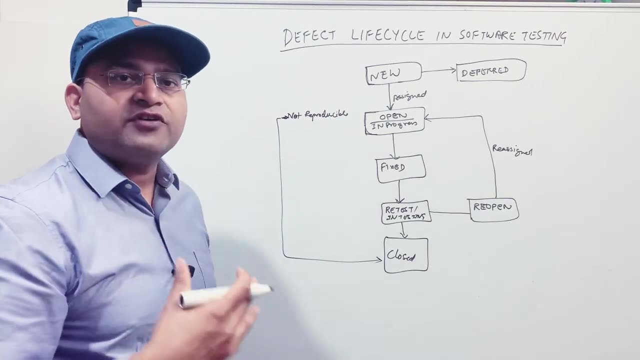 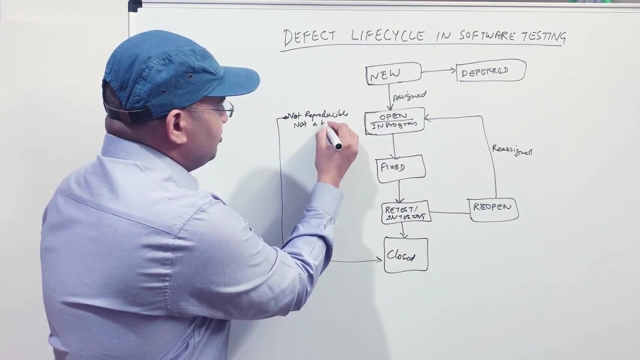 be. if say, for example, the issue was because of the test data. it's nothing related to coding. so in that particular case, if he used proper data and he found that everything is working as as expected, then he will mark it as not a bug. that's another resolution. okay, another could be. 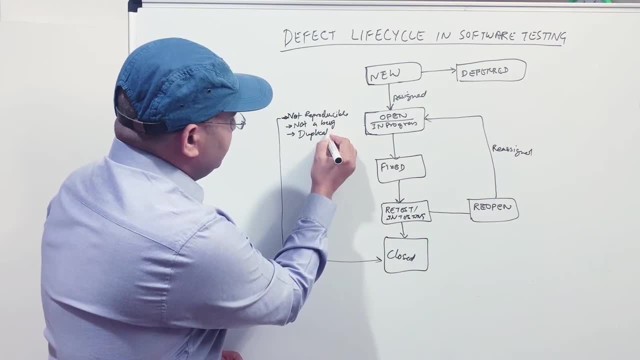 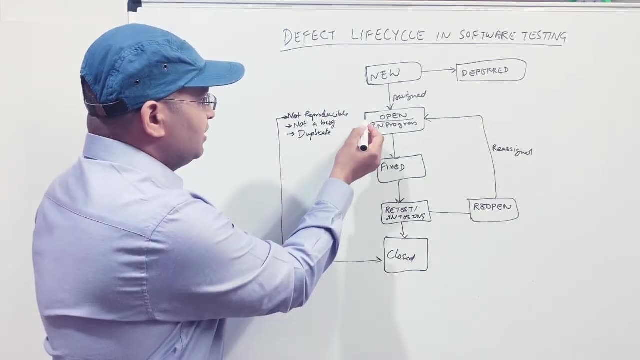 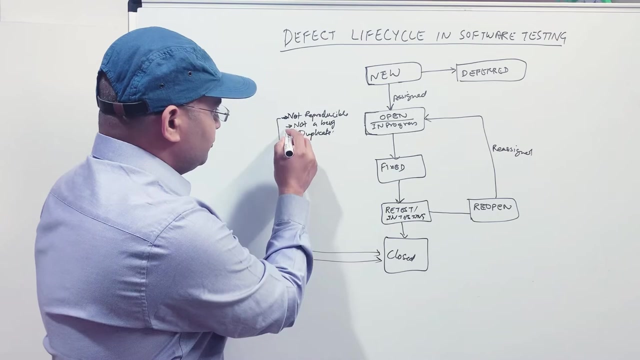 duplicate right. so if there is a defect that you have raised and that a similar defect has been raised prior to this particular defect, during the analysis is found that the defect is duplicate, we will mark the resolution as duplicate and then move the defect to closed right. so this, this flow, is possible as well in 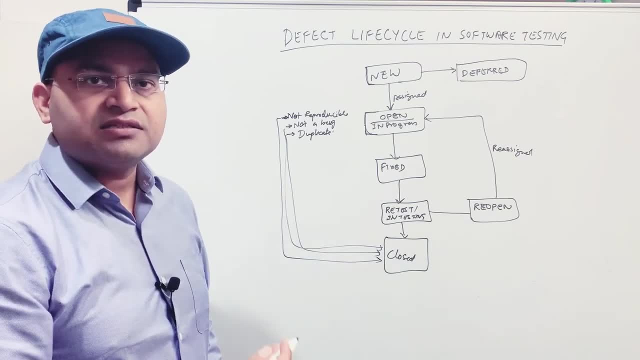 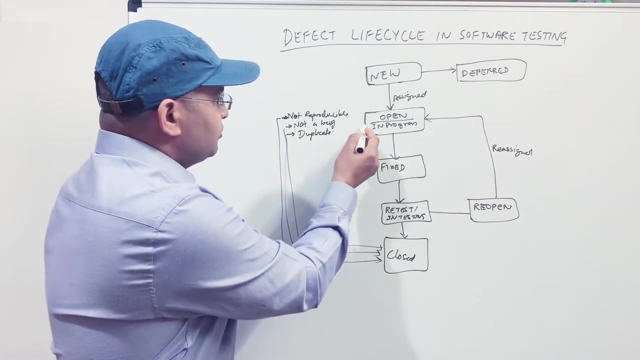 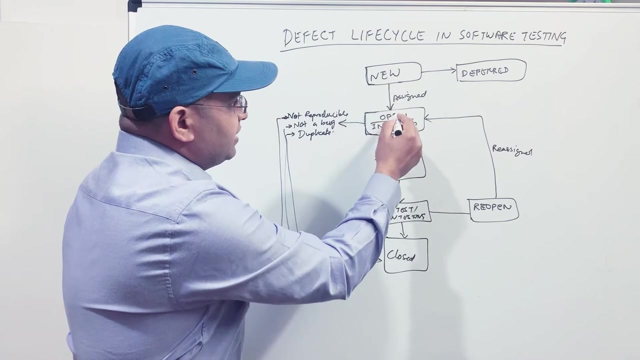 case the defect. during the defect analysis, developer found that defect is not reproducible, not a bug or duplicate of an existing bug. okay, so that flow is possible as well. this is the positive flow. when the defect has been raised- so new defect, then it will be assigned and then, after assigning, developer will. 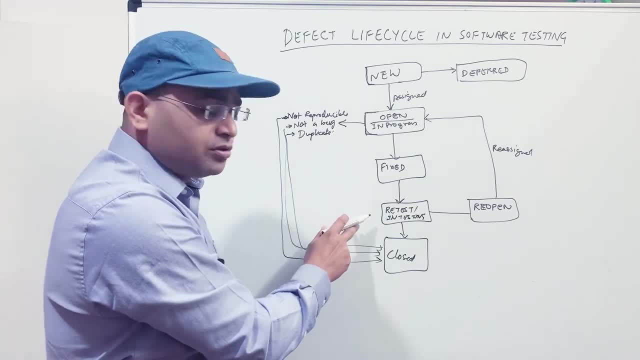 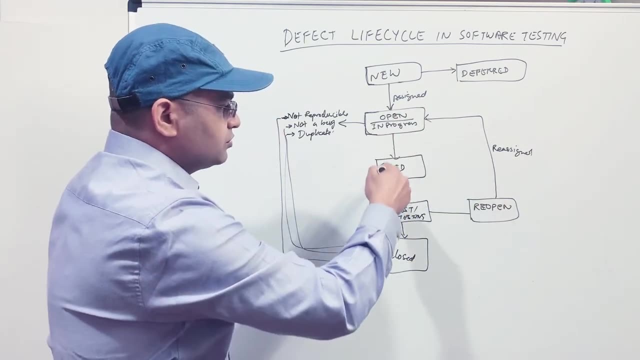 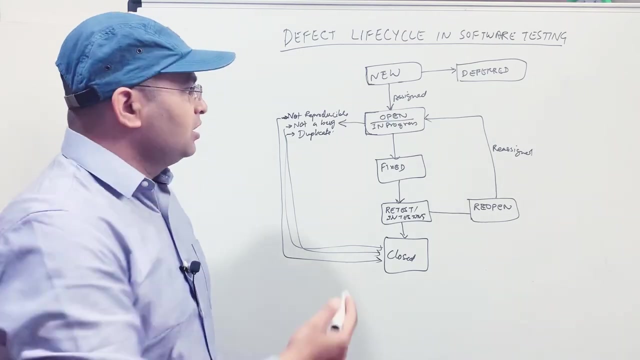 analyze, he'll fix it. you will retest as a software tester. if retest passes, you will close the defect. if retesting fail, you move it to reopen state and it again follows the same process, right? so this is how the defect lifecycle looks like in any software testing project. now 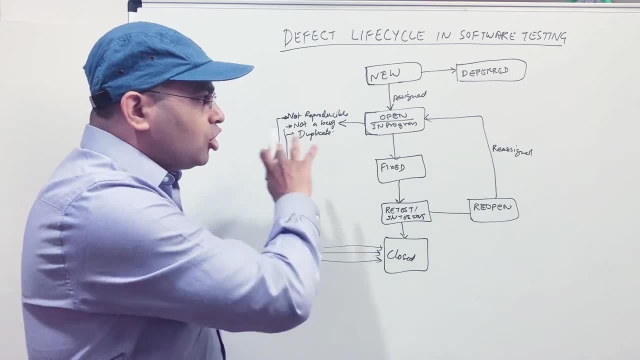 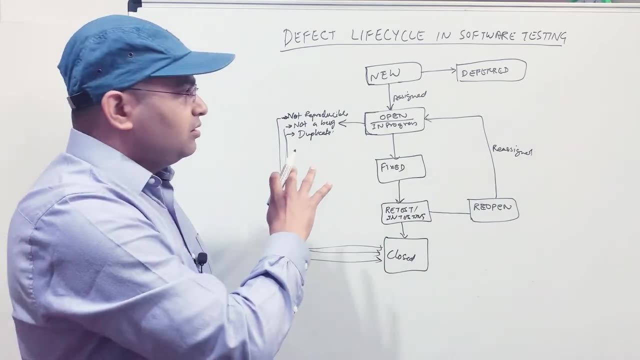 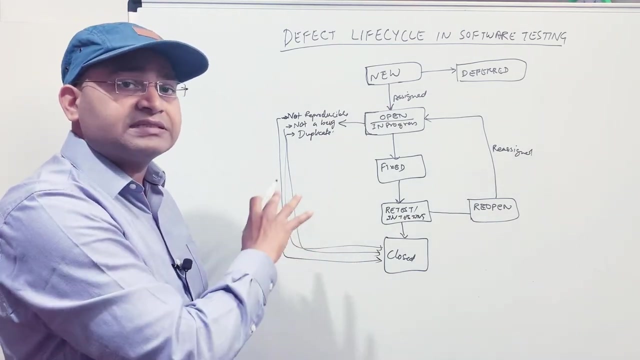 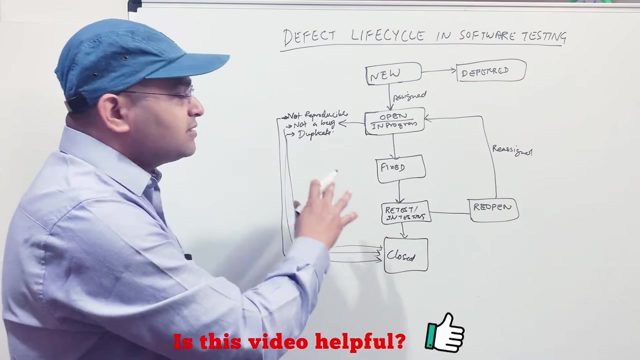 this defect- lifecycle- is common across any you you go into any project, you will find all these states and statuses and resolutions, most of the time in the organization's. along with these resolutions and statuses, there might be requirement within your organization and within your project to have multiple statuses and multiple resolutions extra right. so that is. 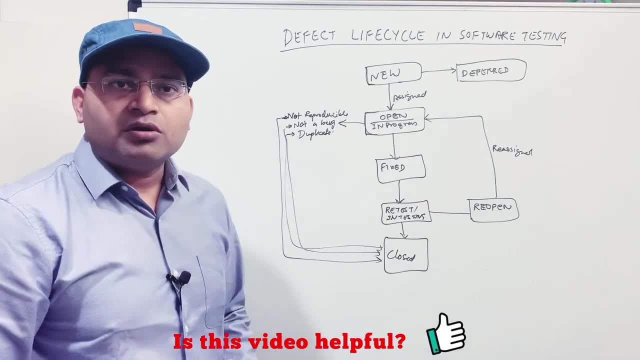 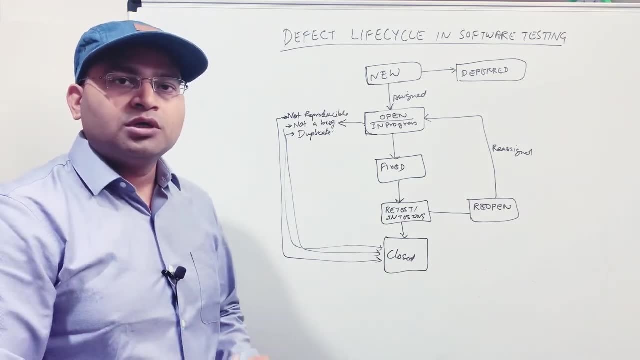 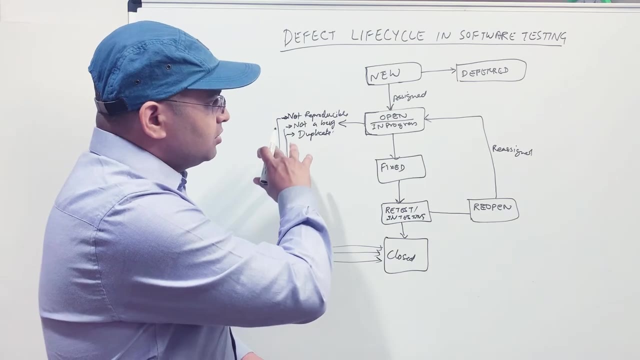 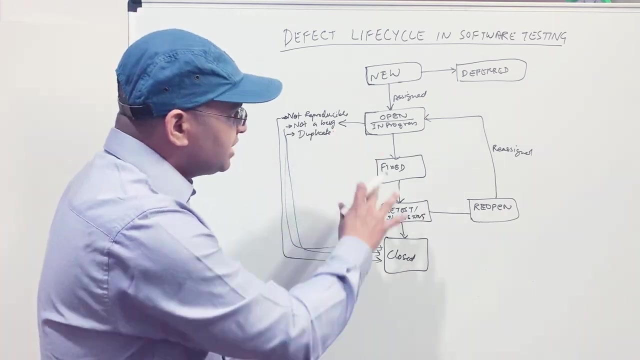 possible because this specific lifecycle is not, is it's. it doesn't fit same to all the organizations. your organization might want to be sick in the, have more granular approach or have not had a multiple statuses and to track defects in a completely different way, so they can customize this. 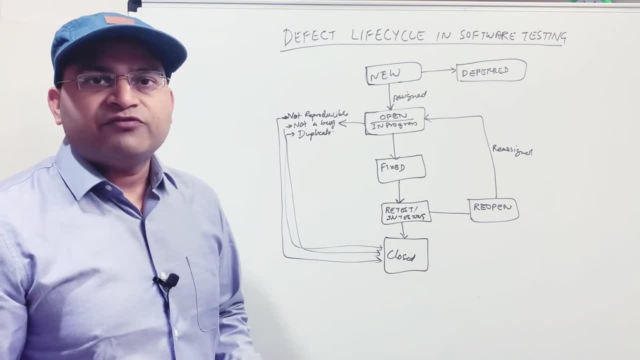 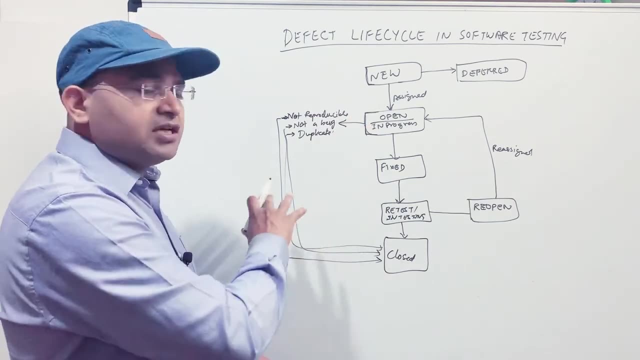 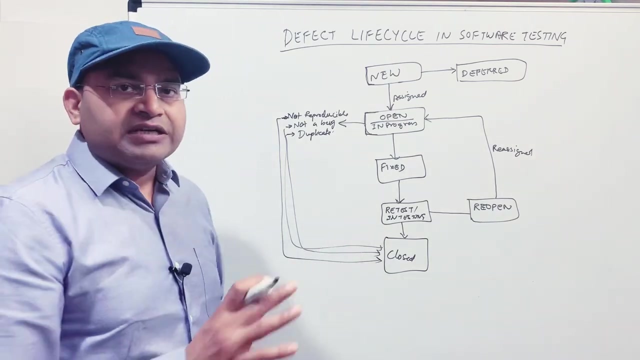 workflow and Jira has built-in defect management functionality, and Jira workflows can be highly customized to enable you to basically have a customized defect workflow as per the project. so do not get worried about the defect workflow that you see, which seems to be very complex or doesn't exactly. 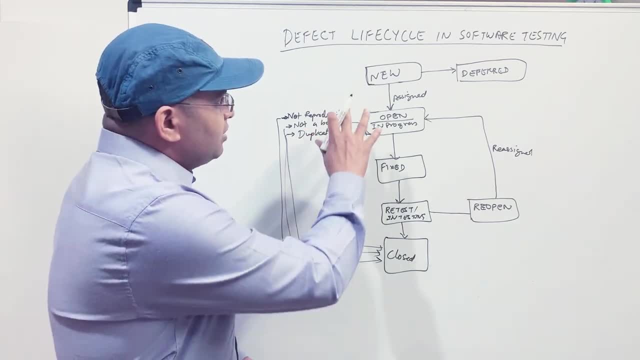 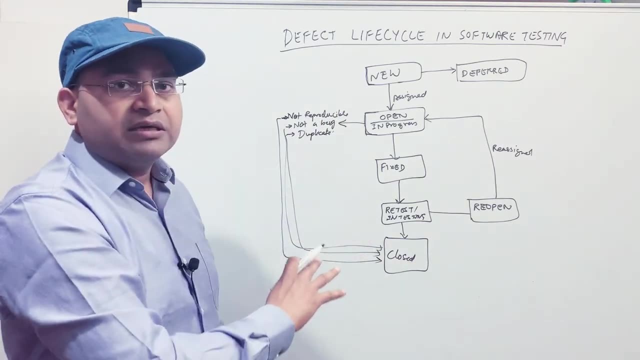 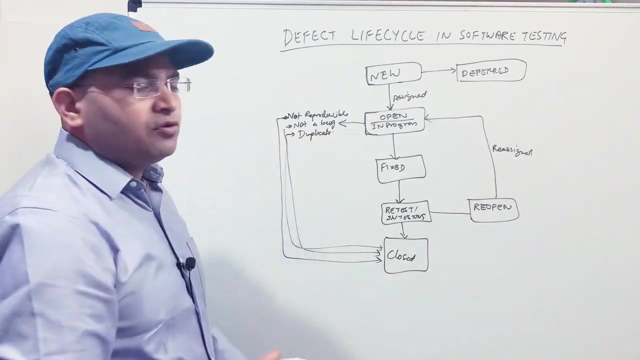 match to this particular defect workflow. however, these are the statuses that will definitely be there in your defect workflow or, most of the time, they will be there in the same form or in some other form. okay, so once you understand the concept of defect lifecycle, how the defect flows, which I have explained in 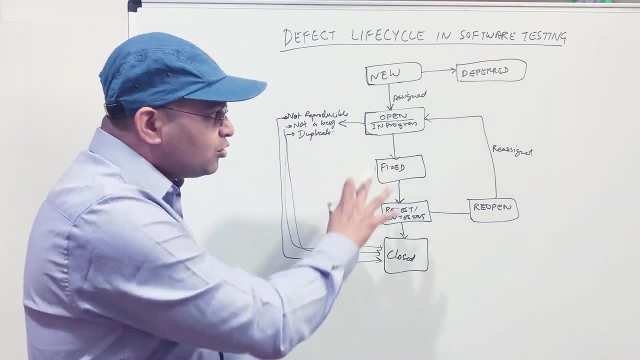 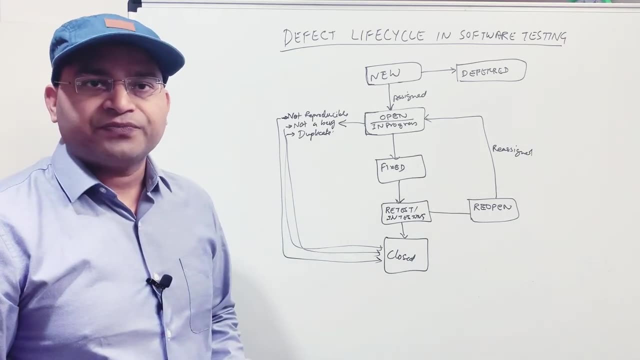 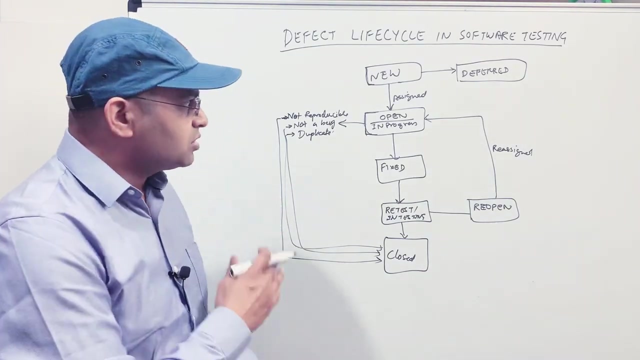 this particular tutorial. practically this is how it will be used, and with some customizations, or a little bit more customizations, or a little bit more customizations, or a little bit more customizations than this. okay, so that's all for this tutorial about the defect lifecycle in software testing. I hope this was clear and you will be clear now. 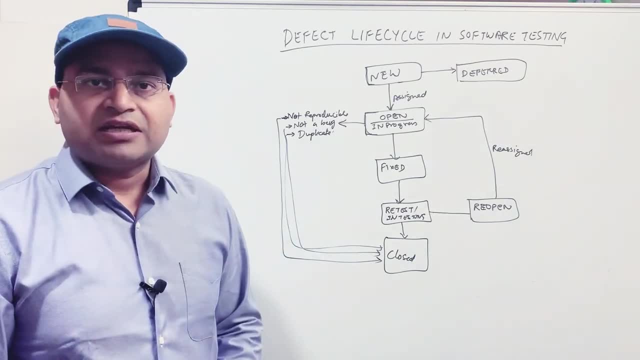 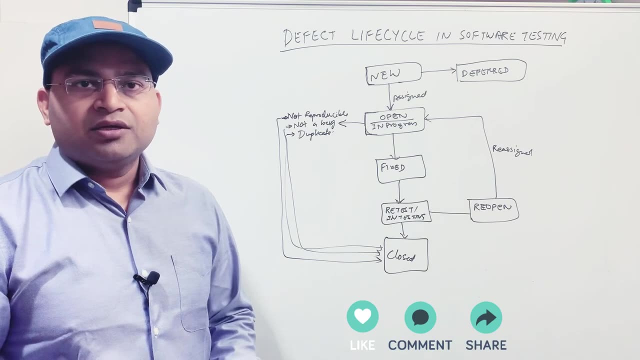 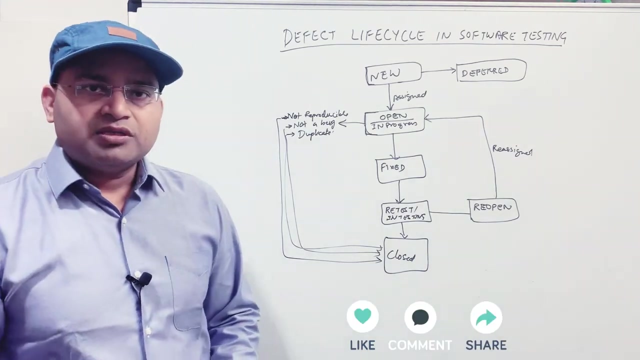 somebody asks you about what is defect lifecycle and explain them about the defect lifecycle so you can explain this along with practical examples, and hopefully you can crack your interview very soon. alright, so that's all for this particular tutorial. thank you very much for watching. thank you.